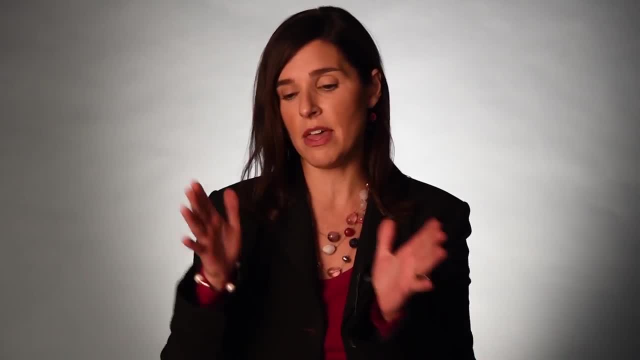 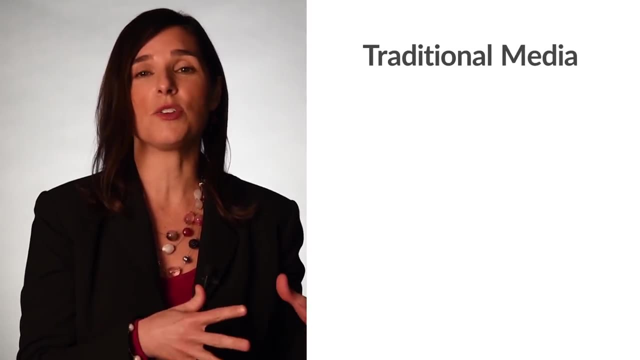 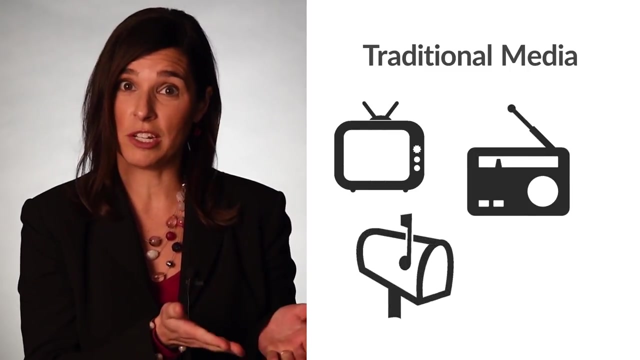 media that you should be aware of. So there's your traditional media, and then there's your non-traditional or new media. So your traditional media is going to be things that you think of like television commercials, radio commercials. maybe it's a direct mail piece, something you find in. 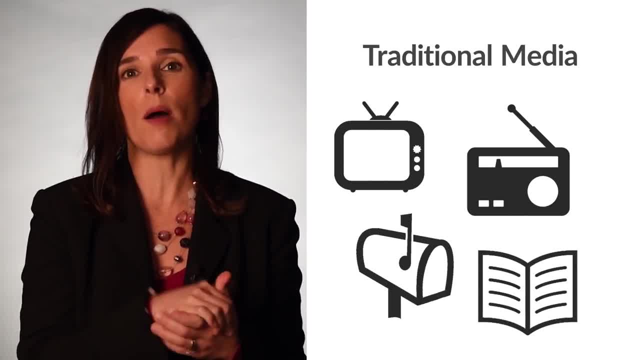 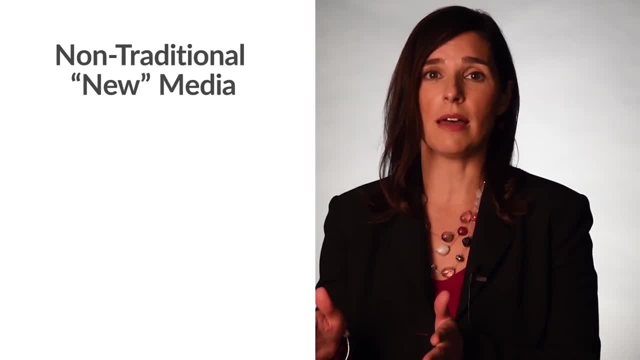 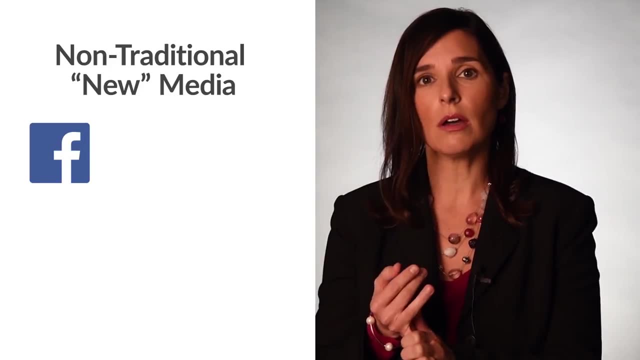 your mailbox. It's a print ad in a magazine or a print ad in a newspaper. That is traditional media. Then, on the other hand, you have non-traditional media and that's the sort of thing that has a platform, an online platform. So, for example, Facebook, Twitter, Pandora, Spotify- any of your 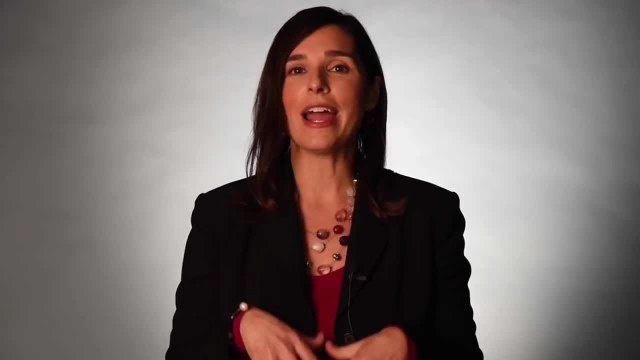 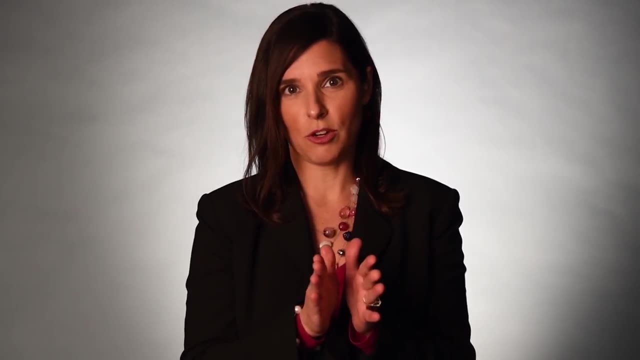 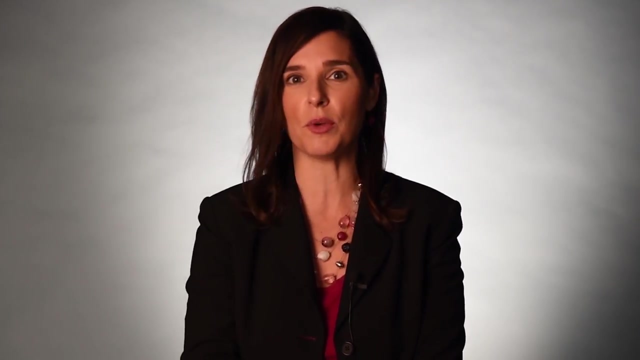 non-traditional new media. Before I dive in to media buying a little bit further, I want to use an analogy, And if you've ever met anybody from Insight Creative, you know that we haven't found a cake yet that we can turn down. So it's going to be a cake analogy. So here we go. When you go to 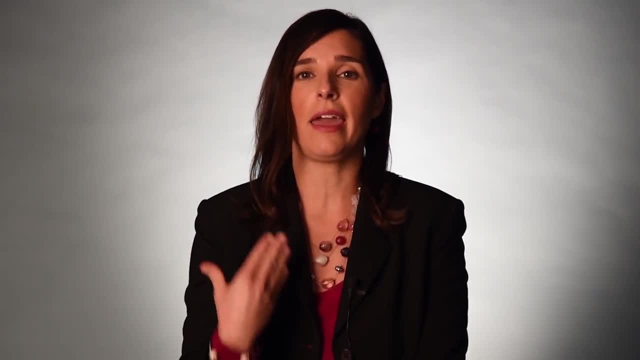 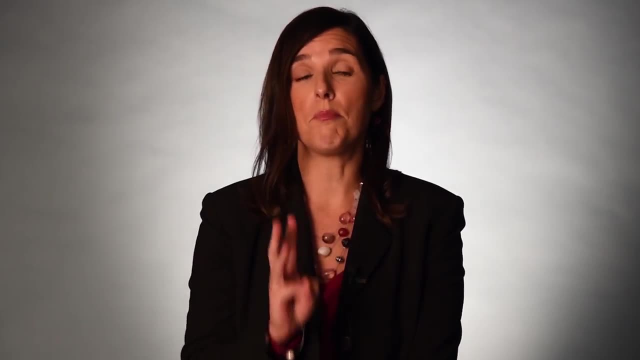 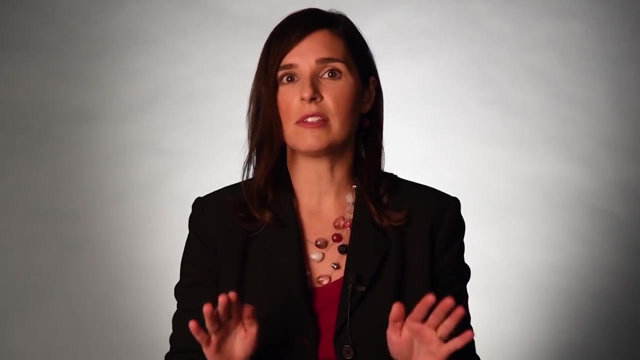 the grocery store and you have it in your mind that you want to make a cake. you go to the grocery store and you buy things like flour, sugar, butter, Oil, eggs. those are all key ingredients to follow this perfect recipe to make a cake. 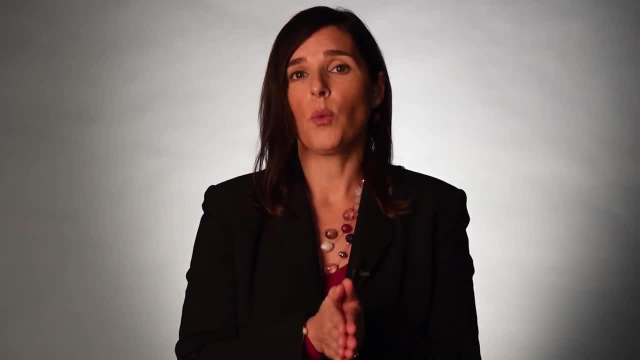 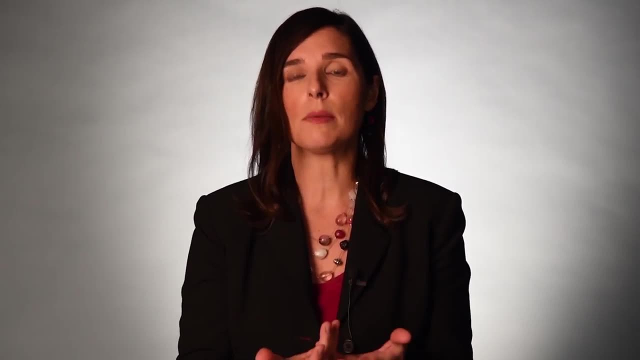 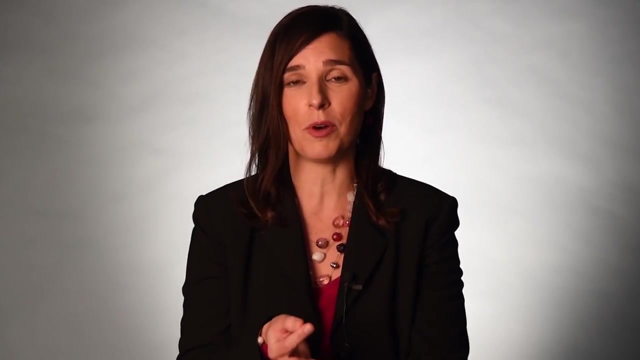 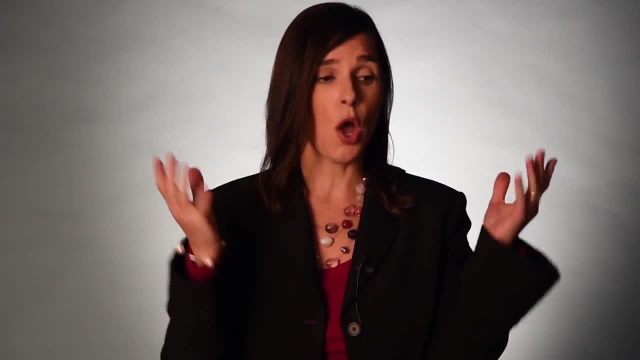 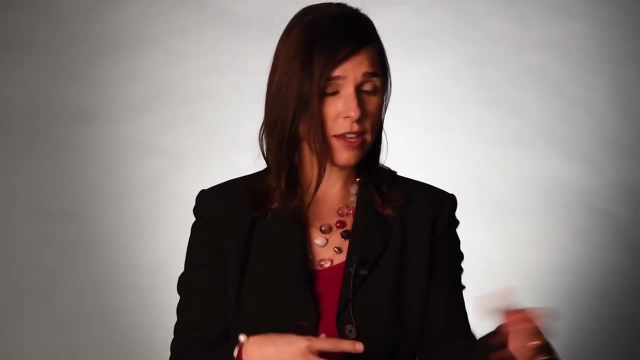 doing this for a long time. I've been doing this for a long time And one of the reasons it's really difficult is because- let's jump back to that cake analogy- when you're walking through the grocery store, people aren't throwing ingredients at you, They're not telling you. you know, buy this or try. 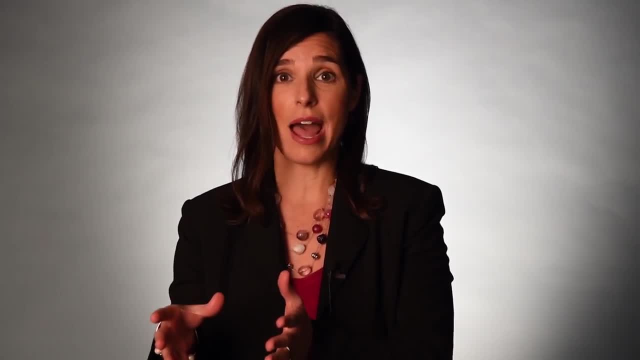 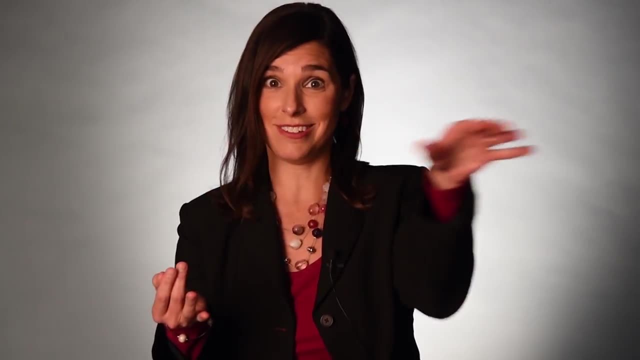 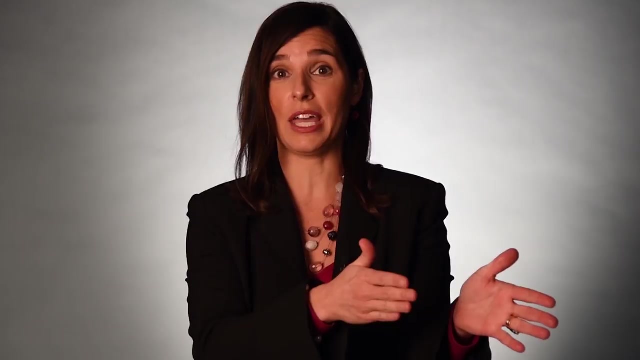 this With advertising. that's exactly what's happening. You don't have the recipe to follow on your own And you have a lot of other vendors, aka ingredients, telling you: use this product, use this service, This is what's right for your campaign, And you don't.